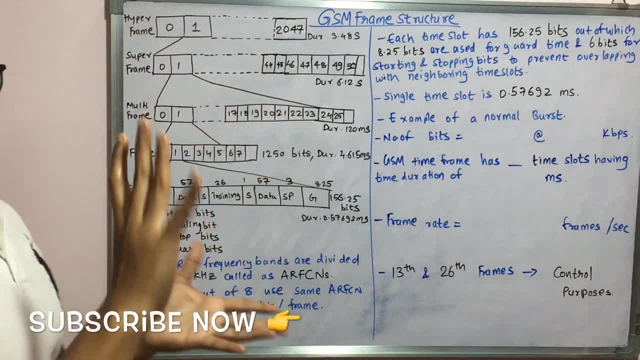 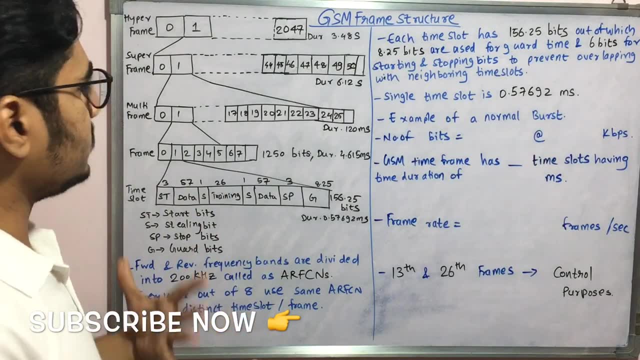 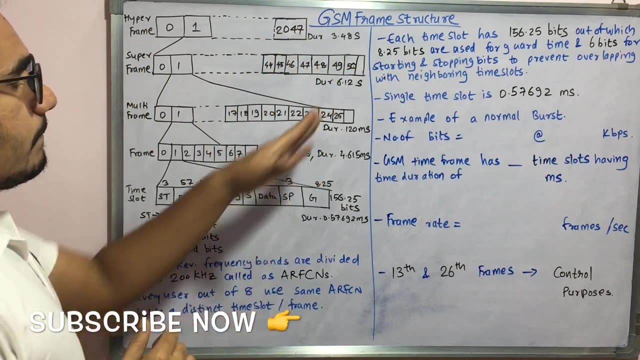 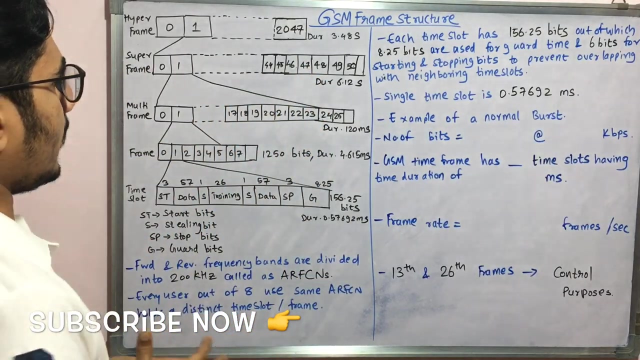 0 to 2047. That is, we have 2048 bits in that And the duration for the entire time frame, that is, for the hyper frame, is 3.48 seconds. Then, when you come down, you have the super frame, which starts from 0 to 50. It extends till 51. And so the entire frame duration for this is 6.12 seconds. Then, finally, you have the multi frame. So multi frame extends from 0 to 25 and extends 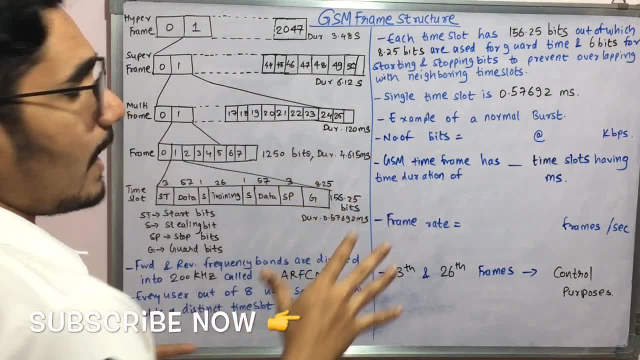 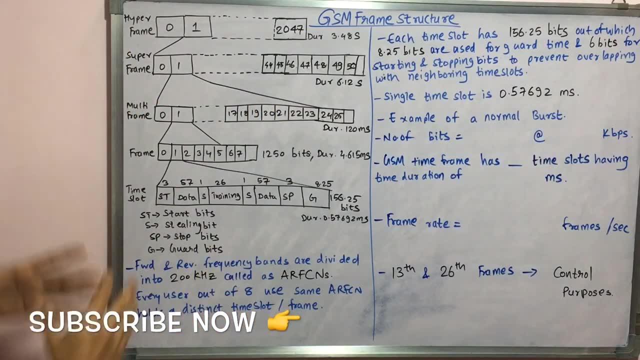 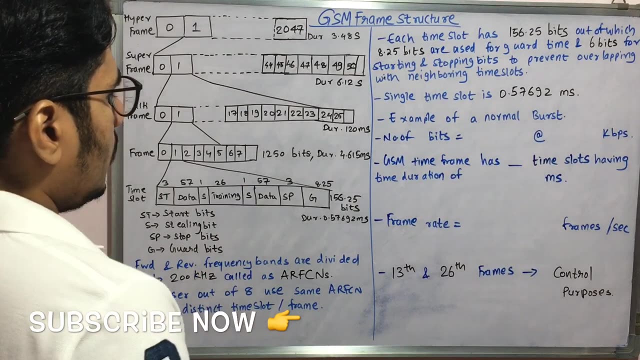 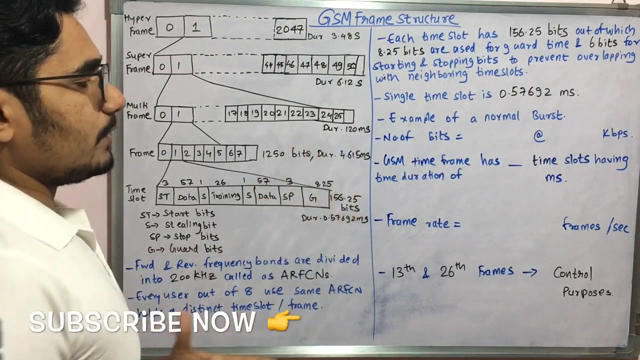 to 1.5 seconds And then when you come down, you have the extra 1 bit is there. that is 26th bit. So you have in total that is 26 bits for that, And so the duration is 120 milliseconds for that. Next, for the frame that is, we have 0 to 7 and extra 1 bit, that is, we have 8 bits in total And it accounts from here till this part. that is 1250 bits in total And the time duration for this is approximately 4.615 milliseconds. Next, we have 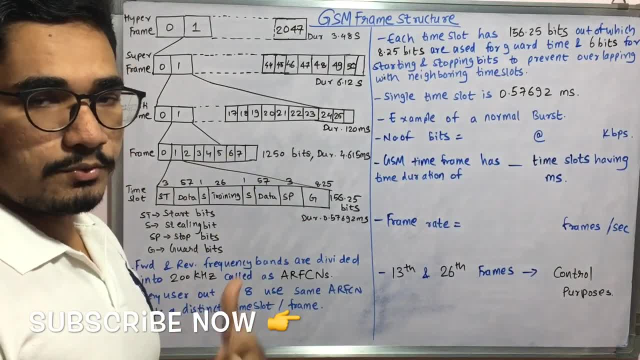 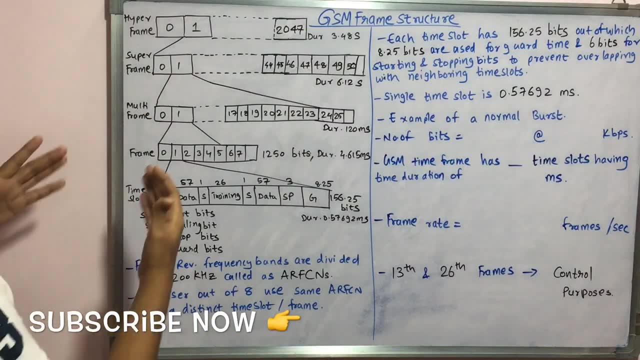 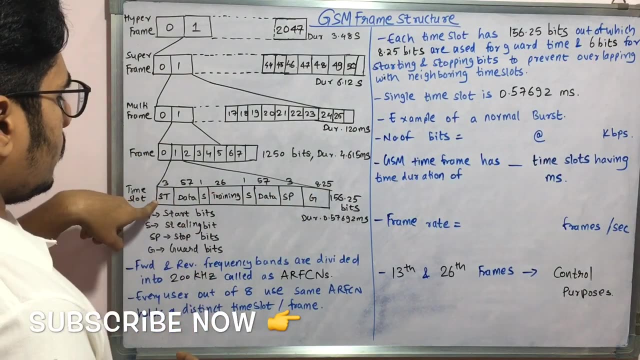 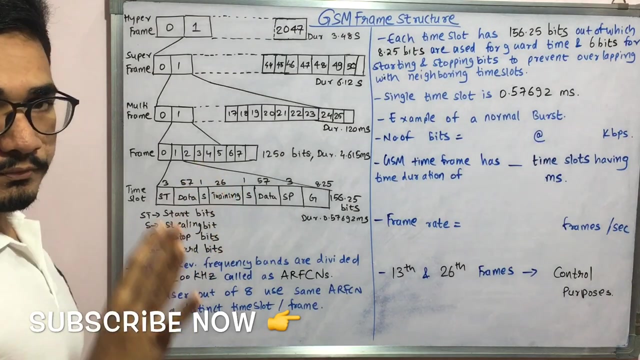 the time slot. So time slot is where the actual data is divided. You can find the flags as well as all the start and stop bits. Also, the data is included in it. So the bifurcation of that bits is something like this: So you have two bits which is start bit, and then you have the stop bit, which is of 3 bits, And then you have the data bit that is of 57 bits And one more data bit which is of 57 bits. Then you have one steel bit which is of 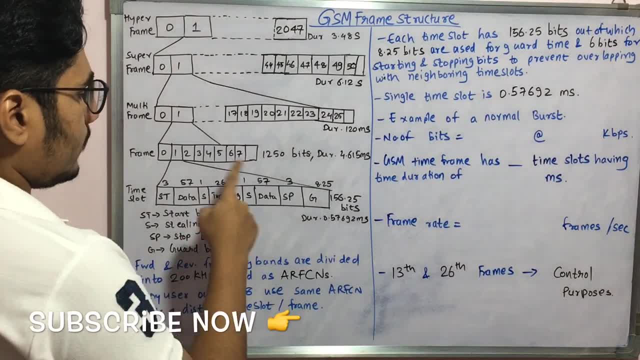 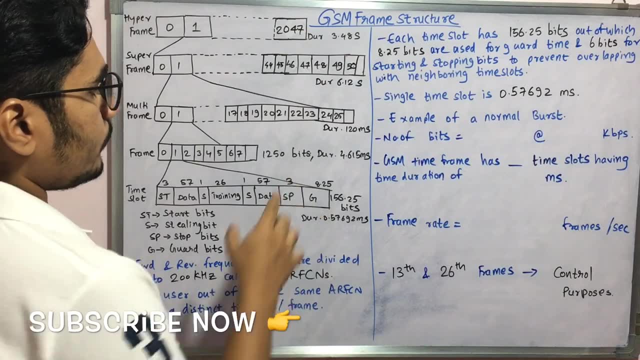 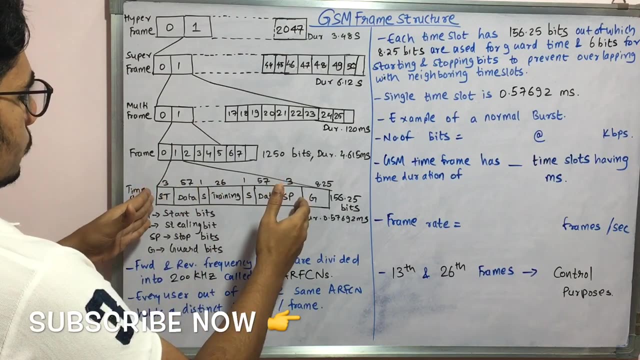 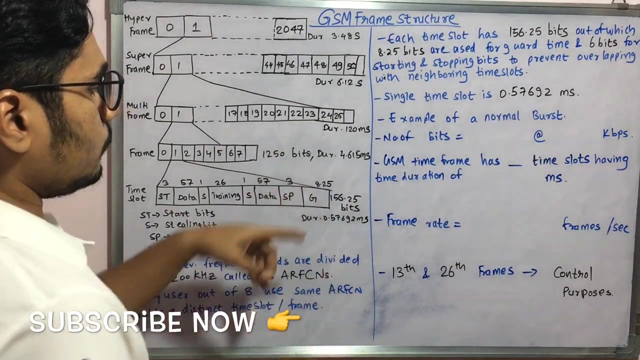 7 bits And followed by you have a training data and followed that you have a stealing bit And finally you have a guard bit for guard time, which is of 8.25 seconds. And so when you just just sum from this 3 to this stop, that is, from this start to this stop, it accounts for 142 bits, And then when you add 8.25- that is guard time- you get a total of 156.25 bits, And the duration for this entire time slot is 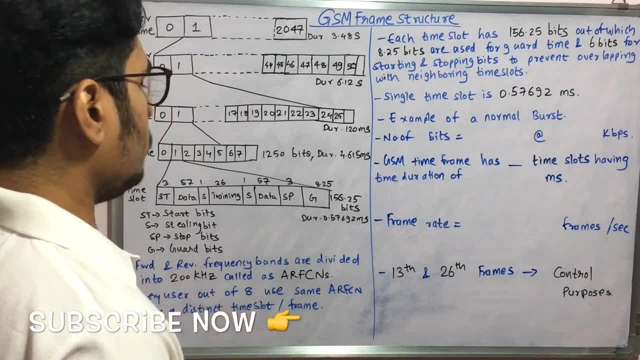 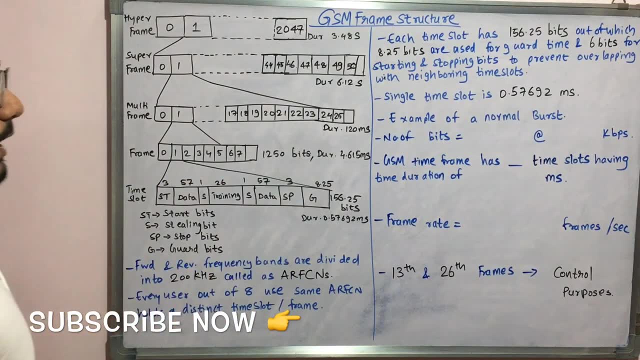 to get transmitted is .57692 in milliseconds, And so this legend is being displayed here, the all the short forms that I spoke. So when we talk about this, in the radio system we saw the ARFCNs, So the forward and reverse frequency bands are divided into 200 kilohertz frequency channel, which is called as: 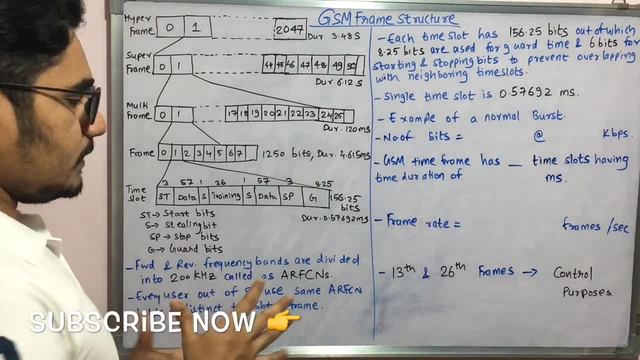 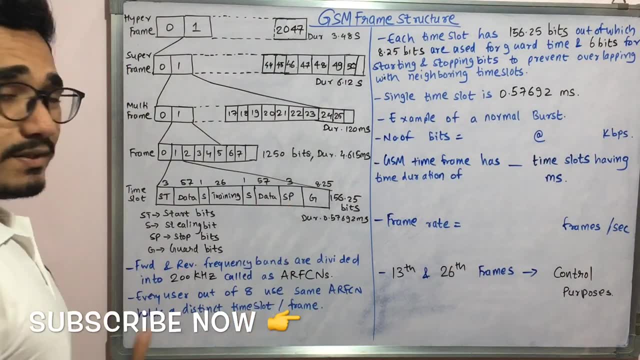 the ARFCNs. Next, every user out of the eight, that is, we have the CDMA users, which allows not to have the ARFCNs. So this sends us a signal that is given as .756 people per minute radio system, that is eight in numbers. they uses the same arfcn and they hold a distinct or a. 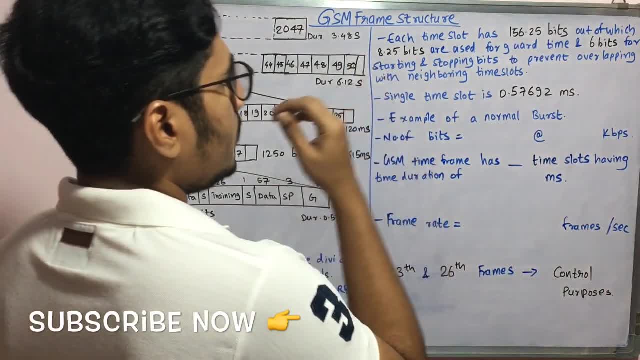 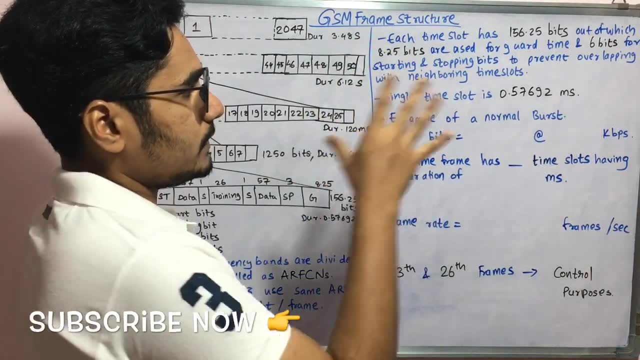 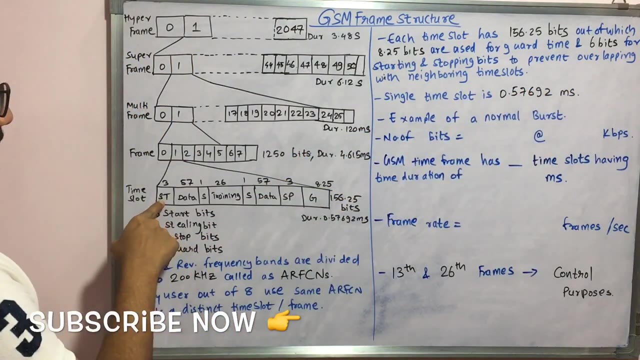 unique time slot per frame. so, uh, now, each time slot in this has got 156.25 bits. that is this one. and from this 156.25 bits, 8.25 bits are used for uh guard time and six bits, that is this uh start. 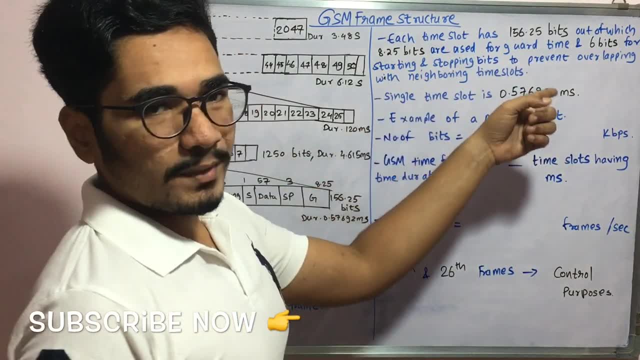 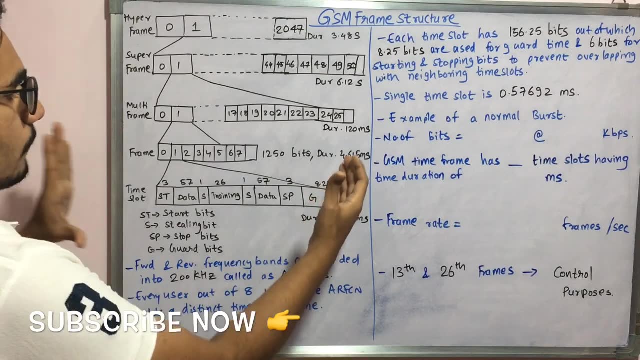 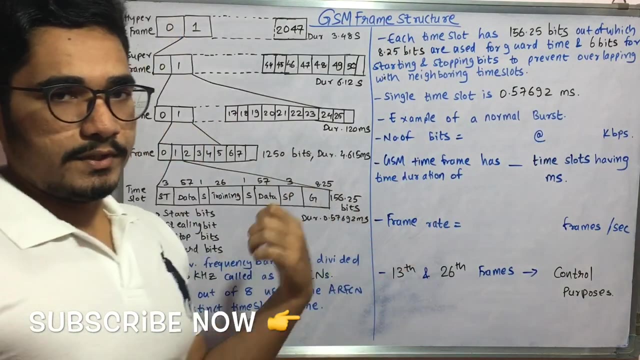 and this top three plus three, that is, six bits, are used to prevent the overlapping which is caused due to the neighboring time slots. so, uh, the single time slot for this one particular frame is about 0.57692. that we saw from this, and so, uh, in this we took an example of a normal burst. now we'll 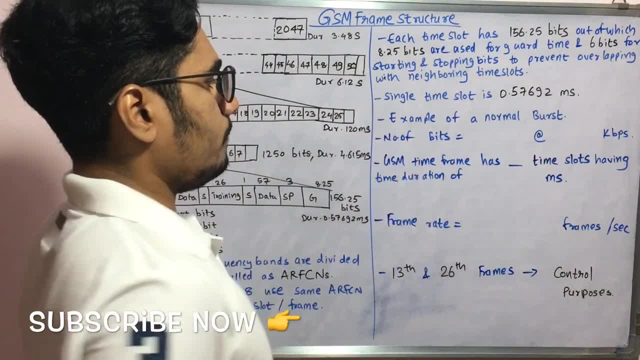 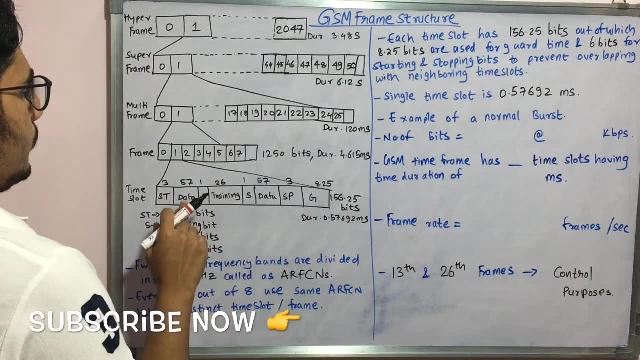 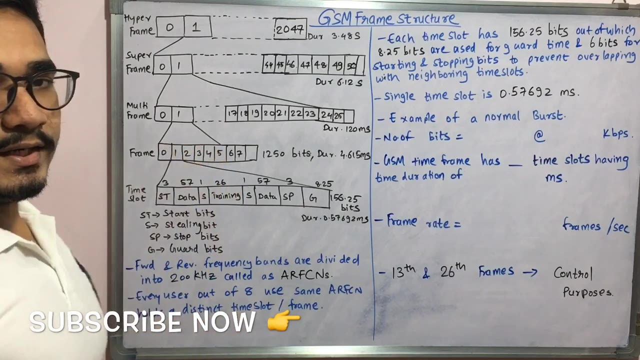 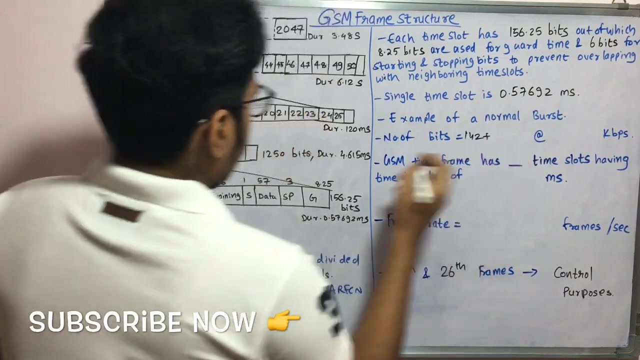 calculate some estimations, that very easy. so the number of bits out of this total, so excluding the uh guard time we have, that is this: we calculate the data that is 57 into 2 times, we have 114. and then you have the training data that is 26. we have 140, uh, then we have 141 and 142, so we have 142. plus this, 3 plus 3, that is 6. so in 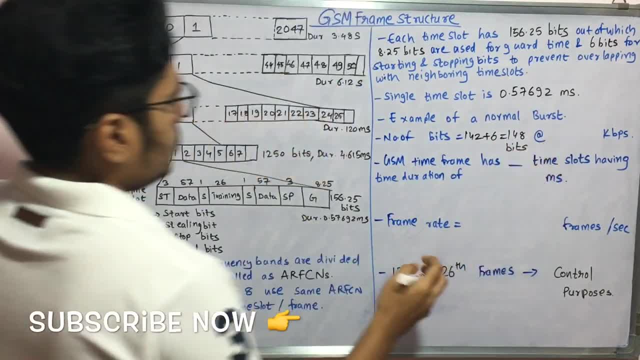 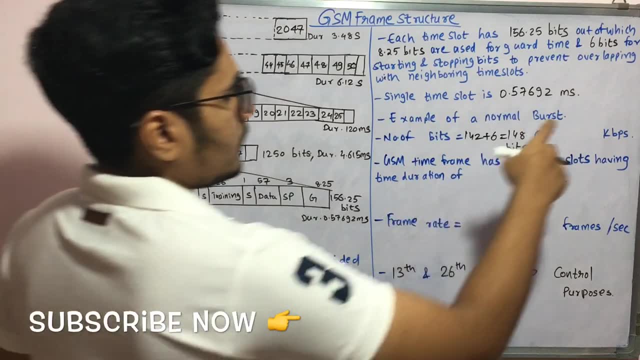 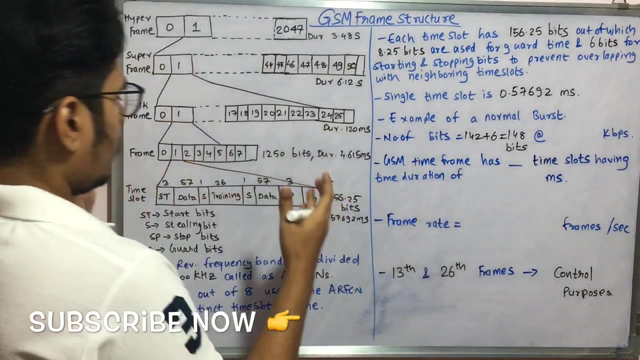 total we have 148 bits in this. so 148 bits we consider in this, that is for this particular single frame and the data rate for this is that will calculate uh from the next step, it's easy. so the gsm time frame, uh, this entire time. 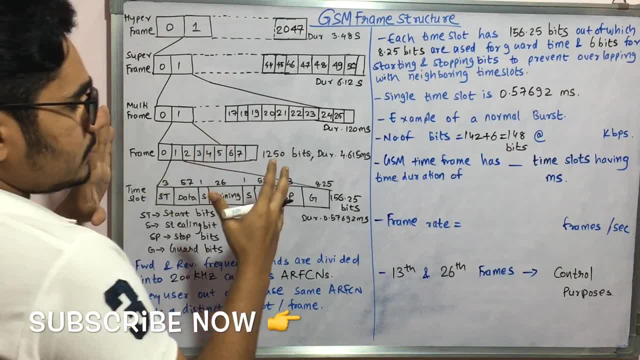 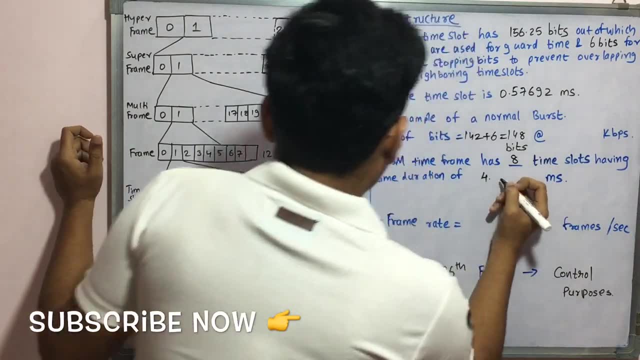 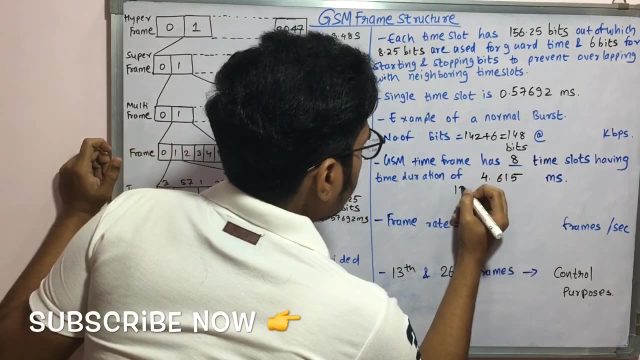 frames, that is, from zero to this seven, so it's a total of eight time slots and having a time duration. uh, that is, we have four point. uh, this one, that is six, one, five milliseconds. so, uh, this time you get from this above. so, uh, when you divide this, 120 milliseconds, divided by that is, we have 0 to 25. 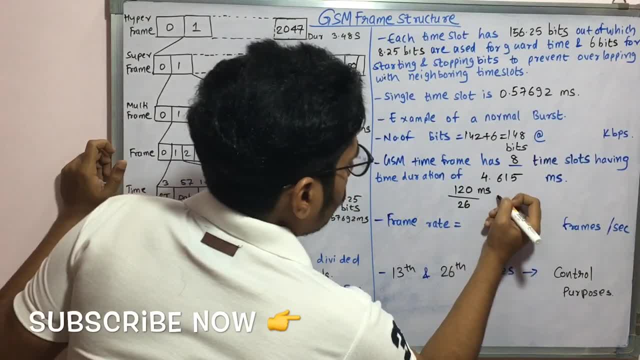 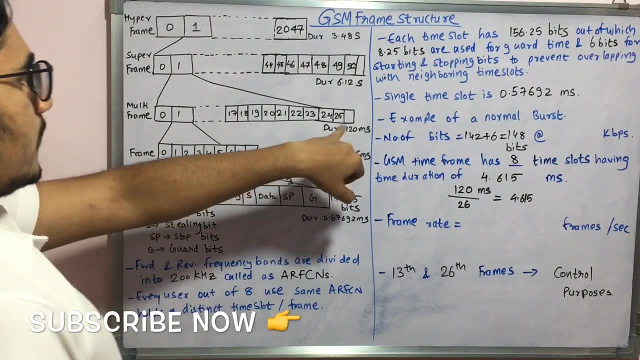 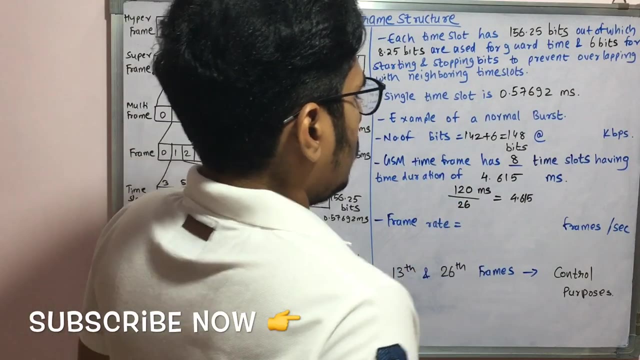 that is, uh, we have 26, so when you divide this and you get this number, that is 4.615. so, uh, the time for this actually gets from the above. that is a multi-frame. since this frame is included in this multi-frame, uh, next for this, uh, we have the frame rate, so before that, we have to write this. 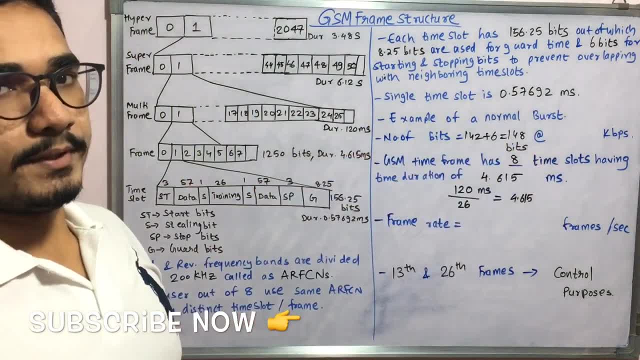 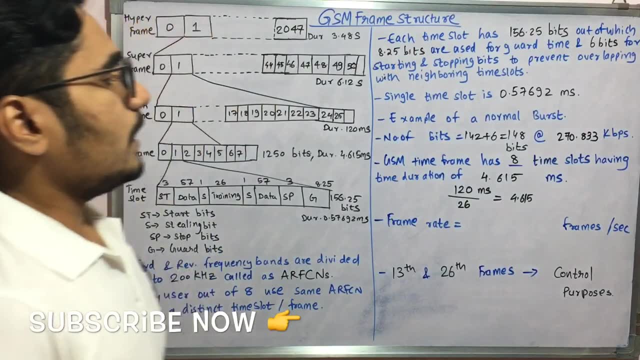 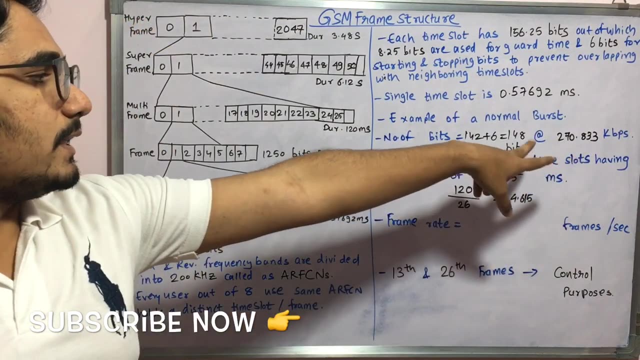 uh calculation, that is number of bits is 148 bits. so 148 bits and the data rate is about 270.7, 0.833 kbps and so it's a standard estimate. we saw in the radius of system so the data transfer rate happens at this speed, that is 1270.833. so that calculation if you uh want to get, so that comes. 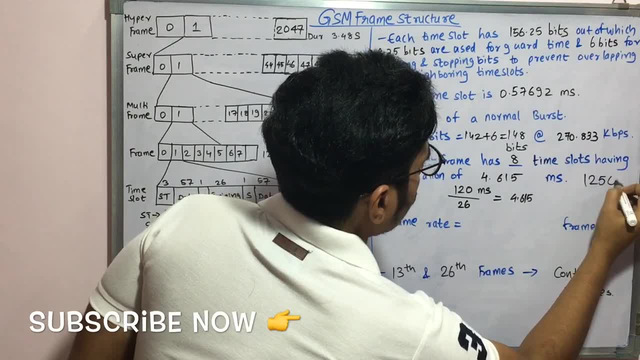 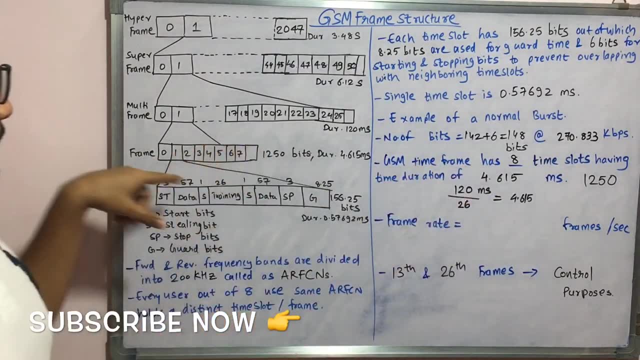 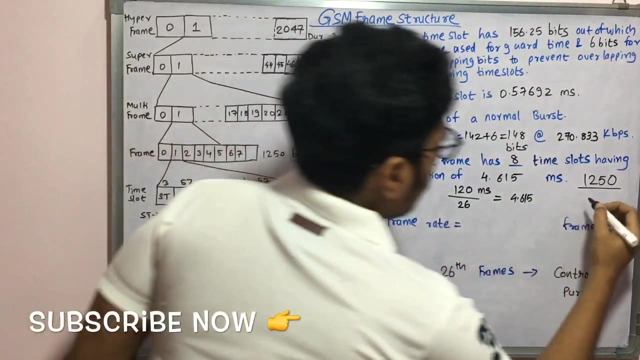 from this number of bits. that is, you have, uh, 1250 bits out of this. so we are just uh, dealing with this frame, that is, we have zero to eight time slots for in this frame and, uh, we have 1250 bits in this and out of this, uh, the entire bit. transmission takes around about 4.615 milliseconds, and so when 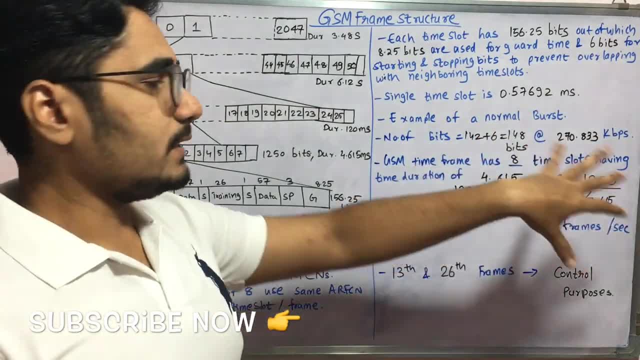 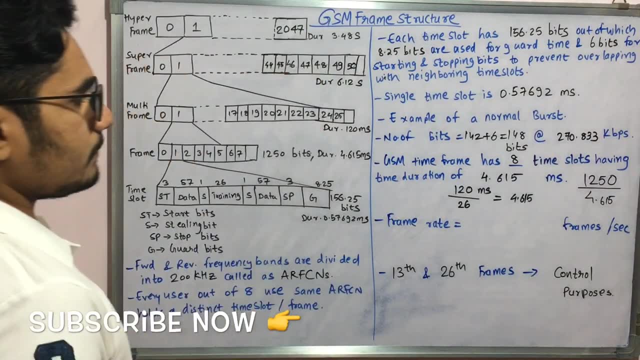 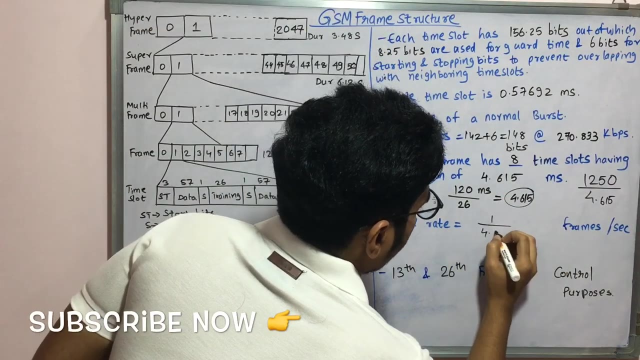 you divide this, you get this value that is 270.833 somewhere. estimation uh with that kbps uh. next we need to calculate the frame rate. so frame rate is nothing but the reciprocal of this time. so if you just uh consider, like uh divided by that is four point six, one five into tender is two minus three. 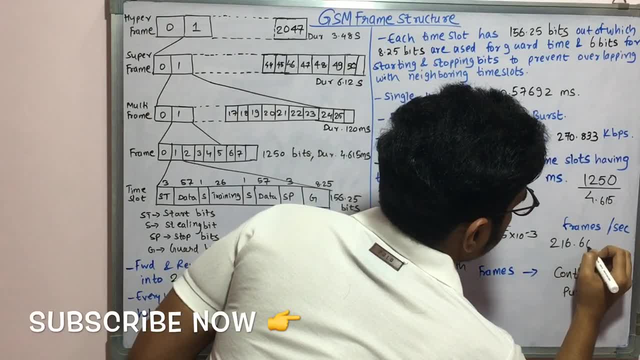 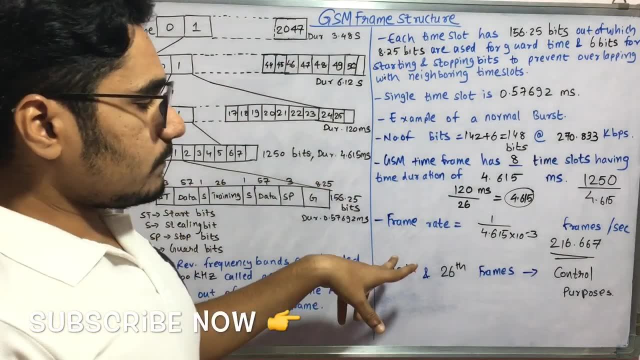 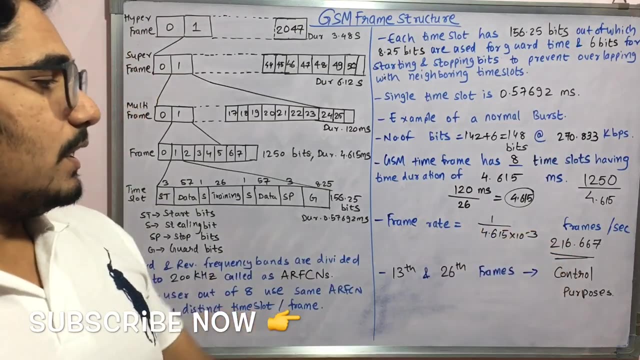 you get this frames per second as 216.667, so this is the frames per second, and then in this entire frame, in each of the frame, each of the 13th and the 26th bits of each of these frames are used for the control purposes, means in the future time it can be used to set as a flag or 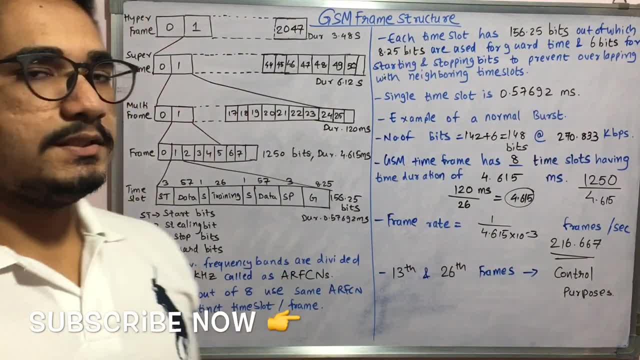 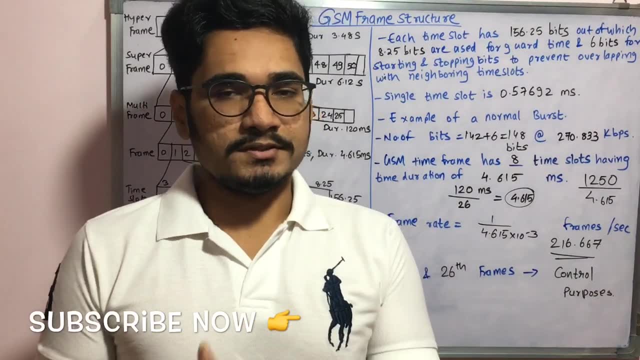 it can be used for any purpose regarding their gsm activity. so well, that was all regarding the frame structures in gsm system, so hope you guys enjoyed this video. if you found it got educated watching this video, please do like, share, comment and if you are new to this channel. please consider do subscribing. thank you very much for watching this video.